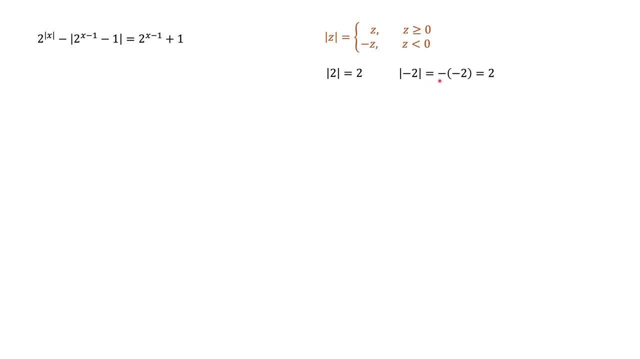 2, minus 2 is negative. the absolute value will be minus of minus 2.. Minus and minus give us plus, and again we get 2, as we expect. So now let's consider the absolute values right here, here and here. So the first one is very easy. we just 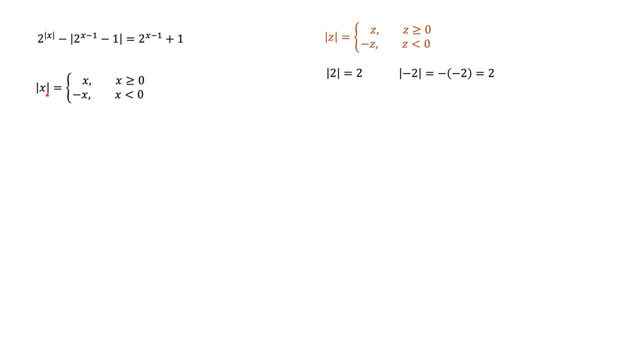 replace Z with X and we get: absolute value of X equals to X when X is positive for 0, or minus X when X is negative. Now, when it comes to absolute value of this guy, we just simply again use this formula and we just take Z as 2 to the power of. 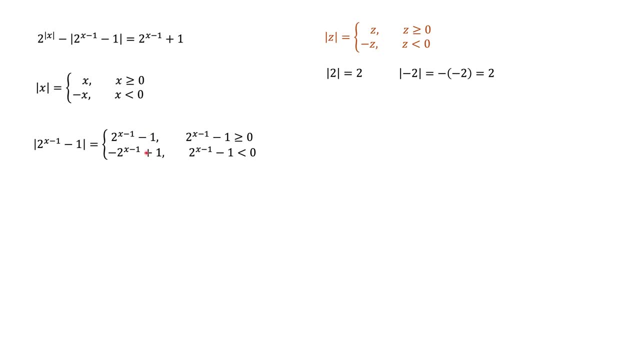 X minus 1 minus 1.. So in this case we can write it like this. but here is a complication. We're saying that absolute value of this complex equals to this complex if this complex is positive for 0 or it equals to minus, that. 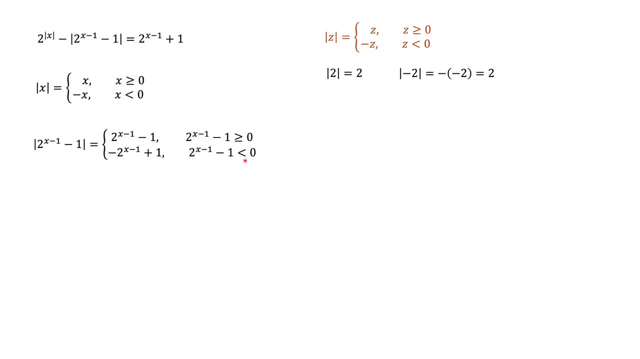 complex if that thing is less than 0.. Now we would like to get rid of these inequalities and convert them into inequalities for X. So to do that, we need to actually resolve this inequality. Let's look at the first inequality. We're going to add 1 to both parts of this inequality. We can do this inequality. 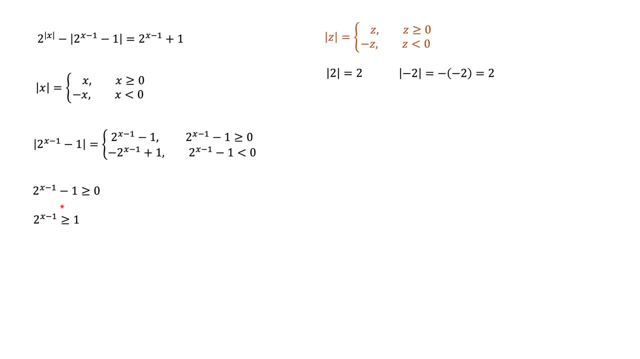 holds. And the next thing: we just need to remember that 1 is 2 to the power of 0. And now we got ourself inequality, where on both sides we have an exponential function with the same base, 2.. On the left, we have 2 to the power of X minus 1.. That's. 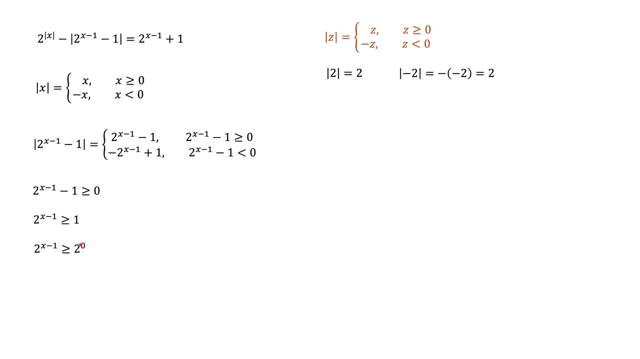 supposed to be greater or equal than 2 to the power of 0. That is possible if, and only if, the arguments of this exponential function, X minus 1, is greater or equal than the argument 0. And that comes from a simple fact that if you 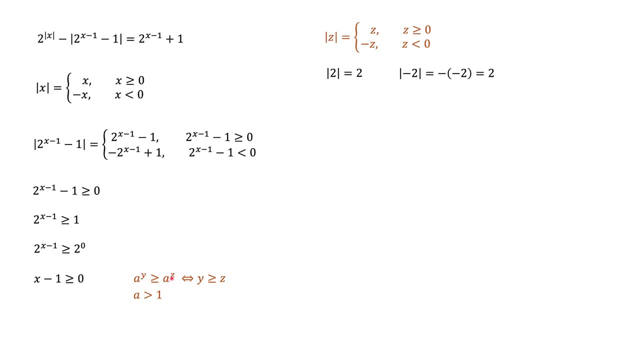 have a to the power of y, greater or equal than a to the power of z and a is greater than 1.. So this relationship is possible if, and only if, y is greater or equal than z And this property falls from the property of exponential functions with a greater. 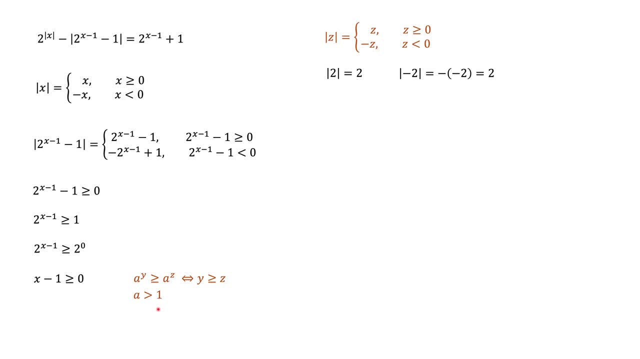 than 1.. But more generally that falls from the fact that exponential function is the base. a greater than 1 is asked monotonically increasing function. And actually there's another video I have when I discuss monotonicity in more details. There's a. 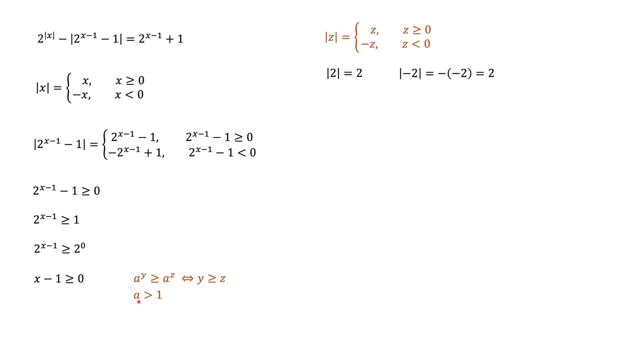 link to it And I'm planning to talk about monotonicity and behavior of monotonic function in near future. So stay tuned. But going back to our inequality, X minus 1 greater or equal than 0 means that X greater or equal than 1.. That means that 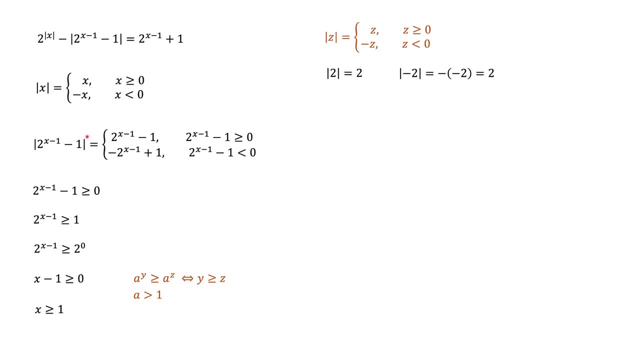 our absolute value term equals to the top expression when X greater or equal than 1, and it's equal to bottom expression if X is less than 1.. So now let's look what we got And that's how we're going to deal with absolute value of X, and that's how we're. 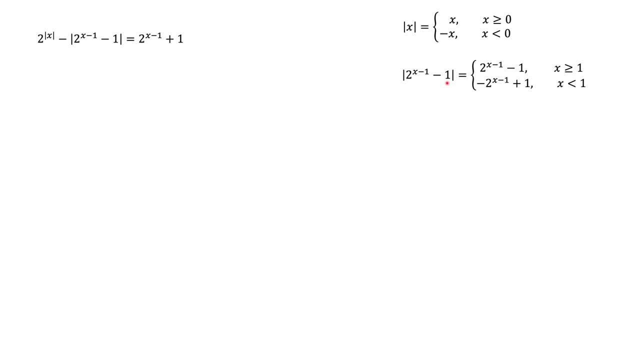 going to deal with absolute value of 2 to the power of X minus 1 minus 1.. So notice that the way the function looks like- absolute values look like- changes when X goes across 0 and across 1.. Essentially, we have three intervals here: X, less than 0, less, greater or equal. 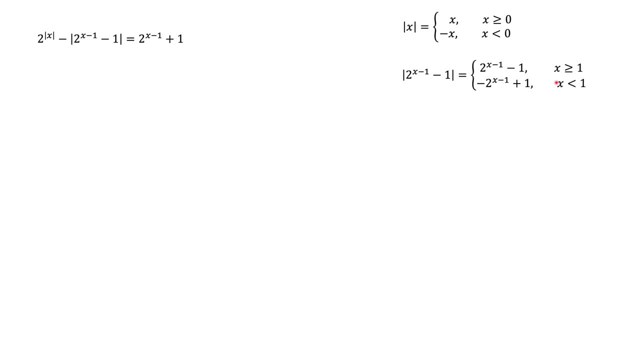 than 0 but less than 1 and X greater than 1.. On each of those intervals, the formula for the absolute values don't change. We start with the case when X less than 1 equals to less than 0. In this case, absolute value of X will be minus X and absolute value of 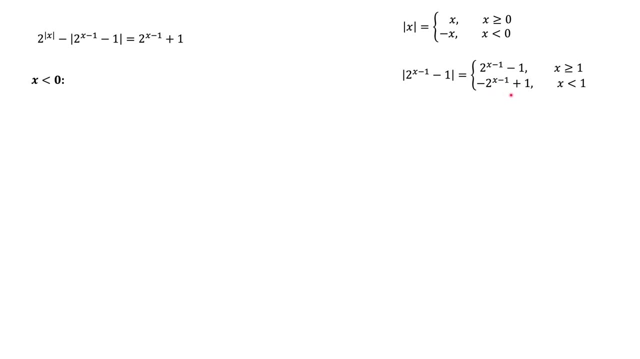 this guy is going to be this guy. So if you plug that in, that's the equation we're going to get. We're going to open the parenthesis and now notice that we have 2 to the power of X minus 1 on both sides of this equation. We can cancel it out And the next thing we're 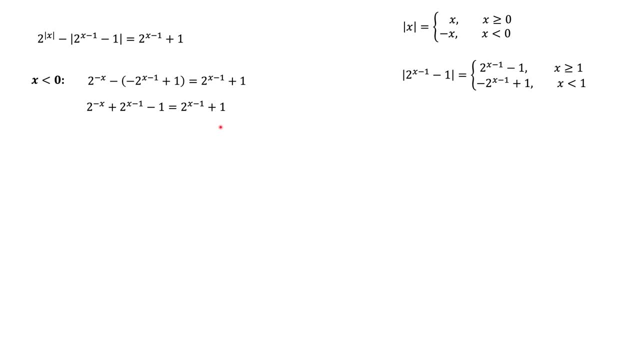 going to do. we're going to add 1 to both parts of this equation. If you do, we get this simple equation. The next thing to notice is that 2 is 2 to the power of 1.. And now we're going to use the following property of exponential functions: If I have A to the 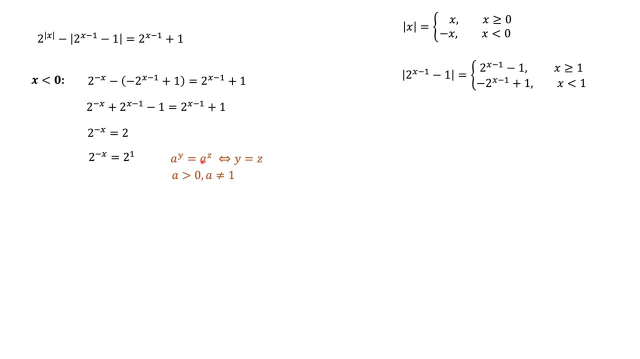 power of Y, which is equal to A, to the power of Z. that is equivalent to saying that Y equals to Z And in our case it means that minus X equals to 1 or X equals to minus 1.. And the last thing we need to check is that really this solution satisfies this condition. 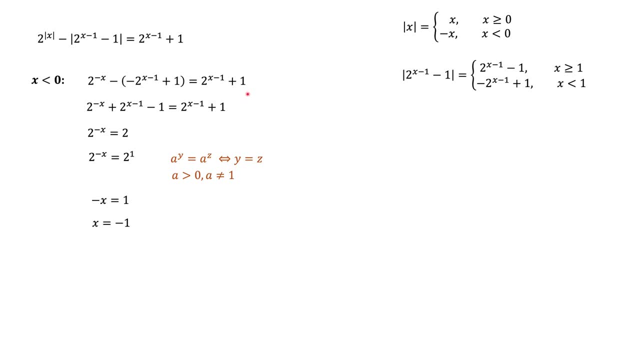 So notice what we did. We solved this equation and that equation gave us this solution, But this equation represents our original equation only in this interval. So the solutions- what we're going to get here- only work if they satisfy this condition, In our case, minus. 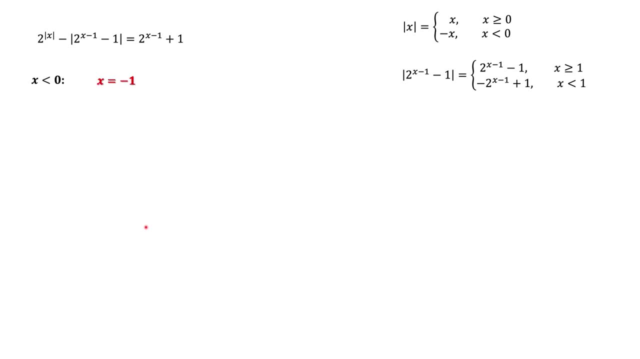 1 is less than 0. So we are good. So X equals to minus 1 is the solution of this equation. The next thing we're going to consider is the next range, from 0 to 1.. In this case, the absolute value of X is going. 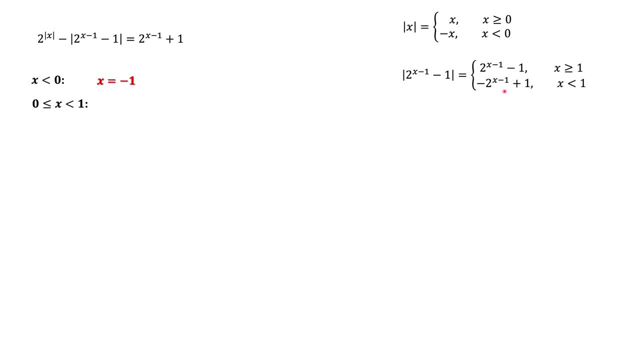 to be X, But the absolute value of this guy is still equal to this. So if you plug that in, this is what we're going to get. We open parenthesis Now again, we cancel out 2 to the X minus 1.. 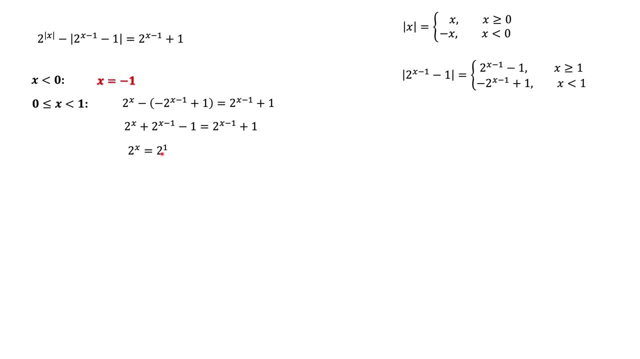 And we get: 2 to the power of X equals 2 to the power of 1, and again, this is only possible when X equals to 1.. And now again we need to check that Dx equals 1 belongs to this interval. And we see that it does not. We see that X does not include 0.1.. So 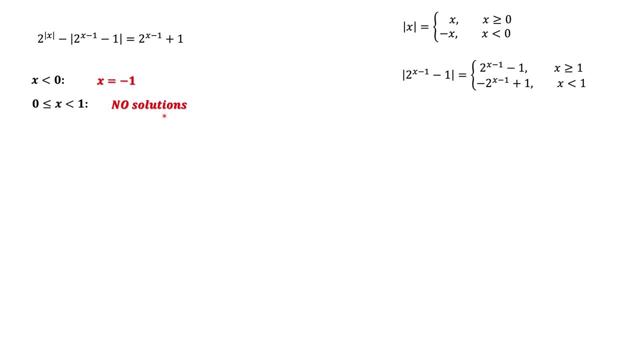 the answer is that in this range we have No solutions. So let's continue and continue understand. Consider the next interval when x greater or equal than 1. In this case, absolute value of x will be x and absolute value of this guy will be the top formula. 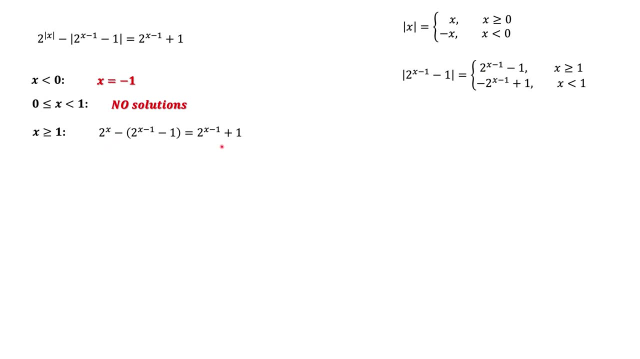 If you plug it in, that's what we get. Open the parentheses here. we're getting this. Now. notice there is plus 1 here and plus 1 here, so we cancel it out And the next thing we're going to do. 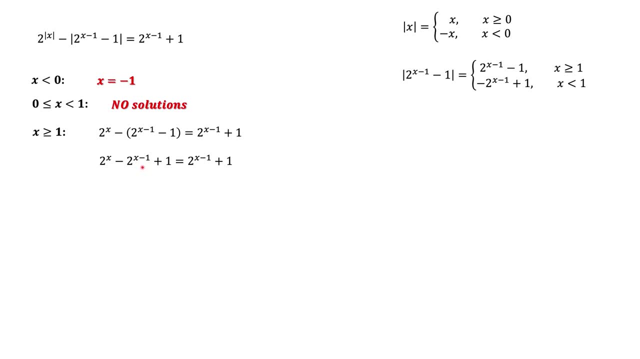 we're going to move this minus 2 to the power of x minus 1 to the right-hand side by adding 2 to the power of x minus 1.. That's what we're going to get. On the right-hand, we have 2 to the power of x minus 1 twice. 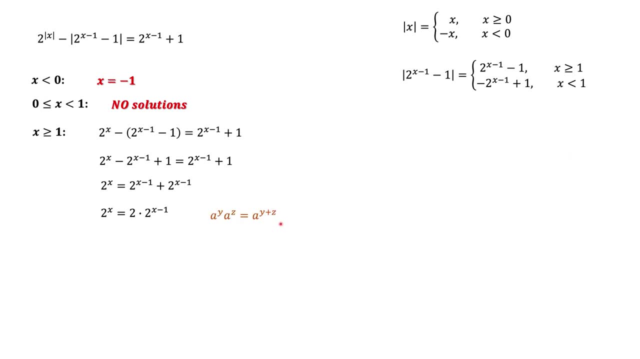 That means this- Now we're going to use this formula for exponential functions- that a to the power of y times a to the power of z equals a to the power of y plus z. a will be 2.. y will be 1, and z will be x minus 1.. 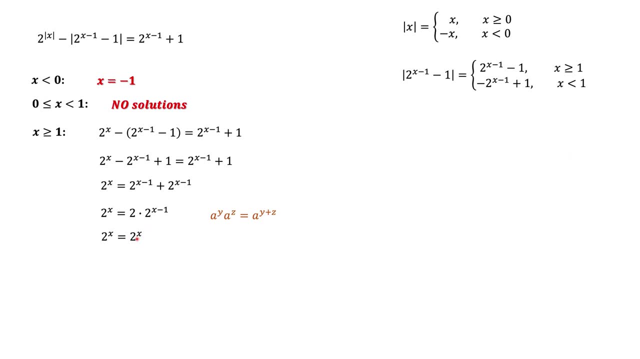 If we apply that, we find that what we have on the right is 2 to the power of x. So now we get a very interesting equation which says 2 to the power of x equals 2 to the power of x. And now the question is: 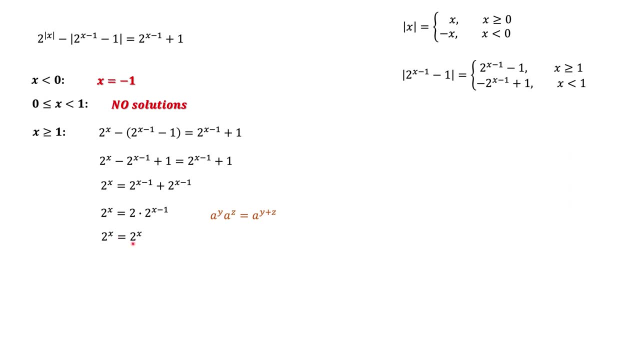 when is this equation satisfied? At what x? And the answer is at any x. Put any x you want you get this equation satisfied. Now we need to be careful before we write that the answer is any x, Because really this solution we got from this equation. 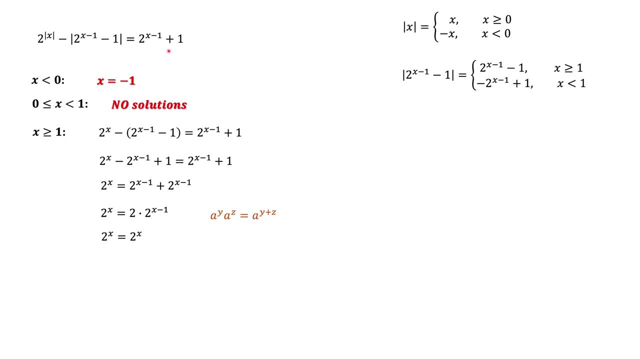 and this equation is a valid representation of our original equation- only for x greater or equal than 1.. So really, when we say any x, we mean any x greater or equal than 1.. So now all we have left is to combine all the solutions. 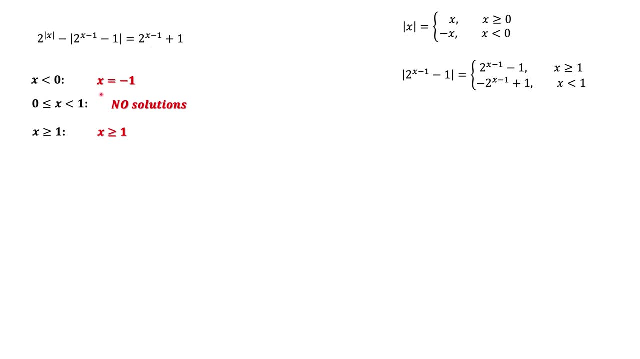 We're going to say that solution of this equation is: x equals 2.. x equals 2 minus 1, and any x greater or equal than 1.. 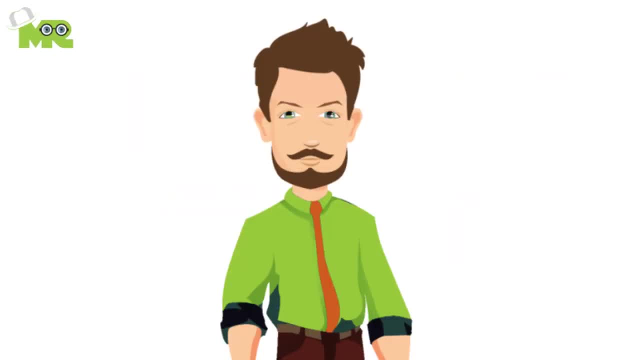 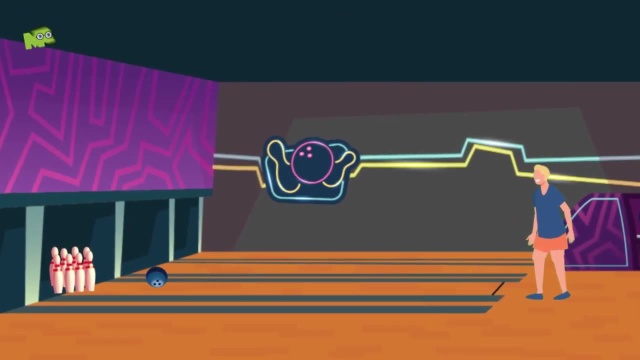 Rules of bowling. Greetings fellow athletes. Today we're talking about bowling rules, So let's start. The objective in bowling: In the game of bowling, the objective is for players to try and score points by knocking down as many pins as possible using the bowling ball. At the end of